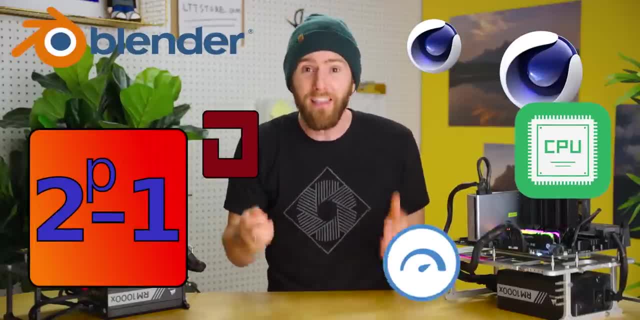 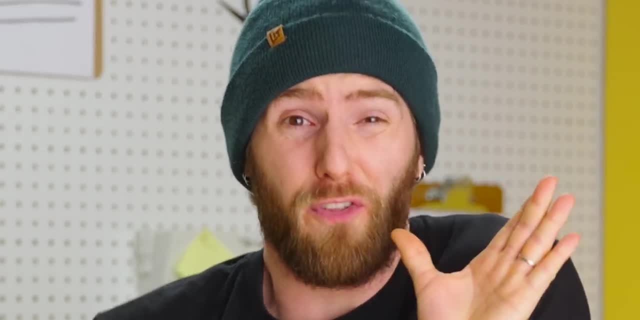 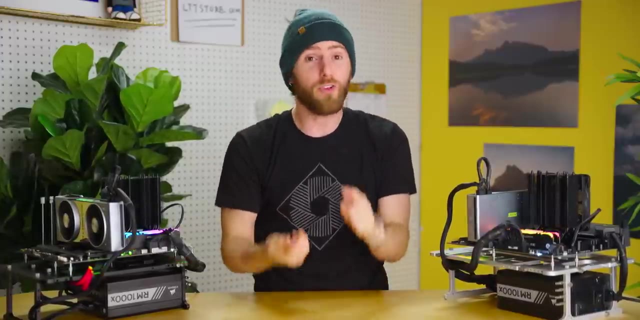 and Cinebench: R23, OCCT Prime95, CPU Expert, Heavy Load, Linux, Intel XT, Ryzen Master, Intel Burn Test, AIDA64, LINPACK Extreme, And that's all just for the CPU. The unfortunate reality is that there is no silver bullet, best test And, depending on your hardware, software and what you're trying to accomplish, you could end up with completely different answers. So yeah, we spoiled the conclusion. Prime95 runs the hottest, but even then, which of the five tests- 10 if you include the AVX2 checkbox- should you run To find out? 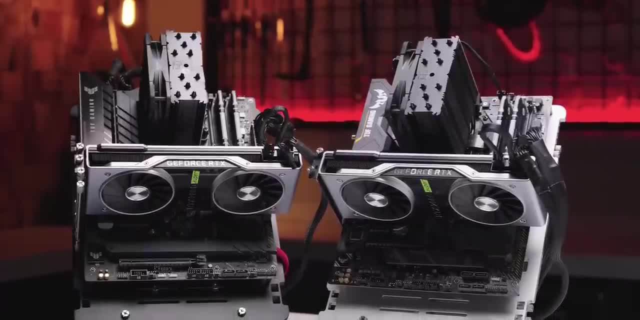 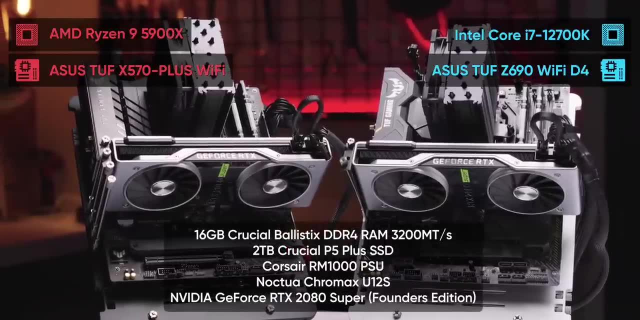 we built up two identical PCs with just two differences: motherboard and CPU. Here's the thing: We suspected that Team Blue and Team Red might behave differently under extreme conditions, and we didn't expect that to be the case. So we built up two identical PCs with just two differences. 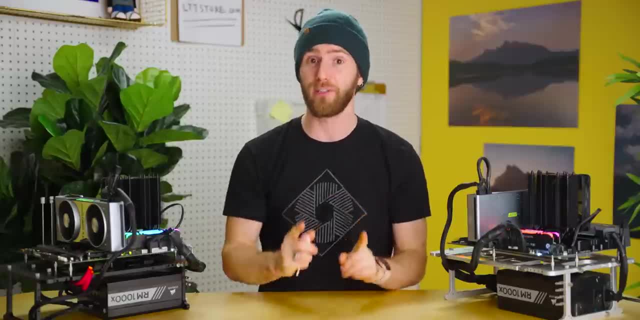 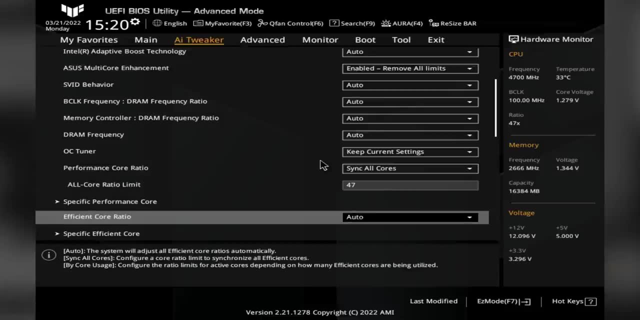 motherboard and CPU. Here's the thing: We suspected that Team Blue and Team Red might behave differently under extreme conditions, and we're really glad we tested both, because they absolutely did On both platforms, though we also locked our CPU clock speeds, core voltages and fan speeds, leaving 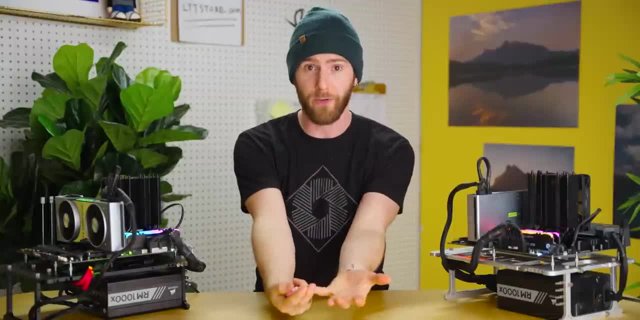 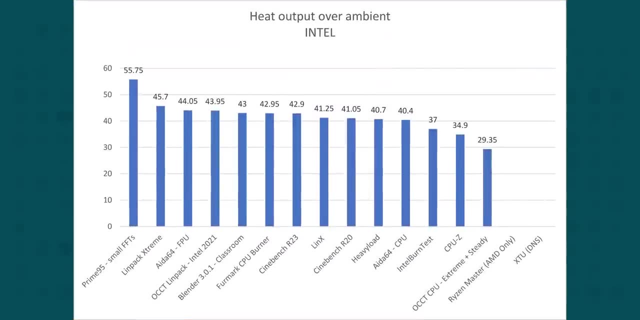 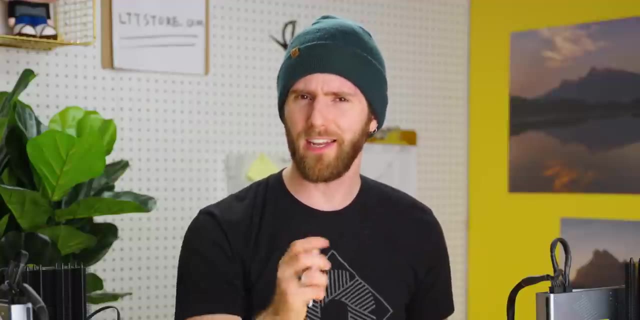 just our CPU temperatures as our stress indicator. Time to show them the graphs. Give them the graph. editor: Intel. first Two tests didn't work at all: Ryzen Master- we saw that one coming- and Intel Extreme Tuning Utility- We didn't see that one coming. It ended up erroring out the same way. 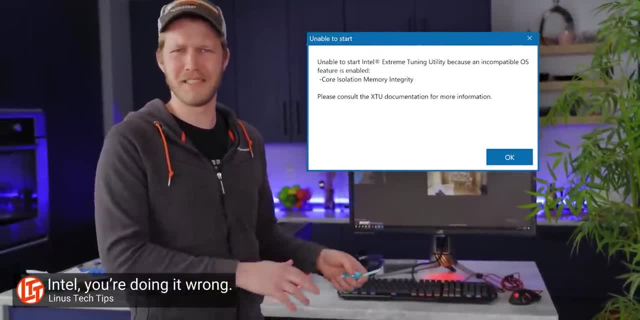 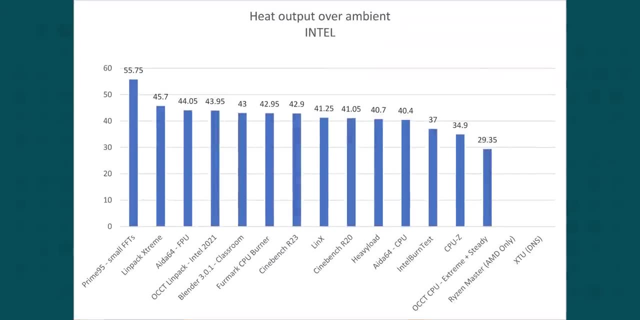 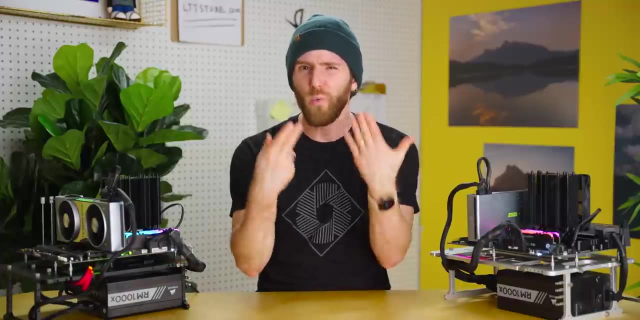 in Windows 11 that we saw in our recent Dragon Canyon Nook video. Among the tests that did work, Prime95 Small FFT stood absolutely alone, beating out the next highest score by 10 freaking degrees. There's just no other way to put this. We did not believe our results, So thinking that maybe Intel's 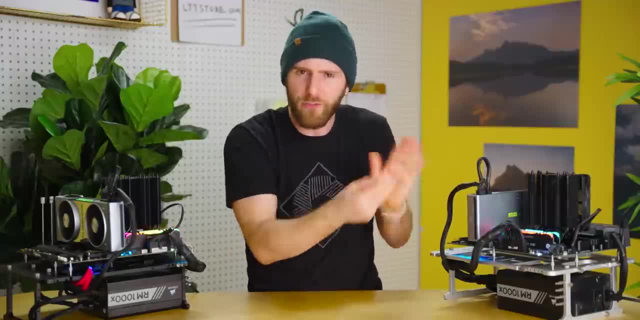 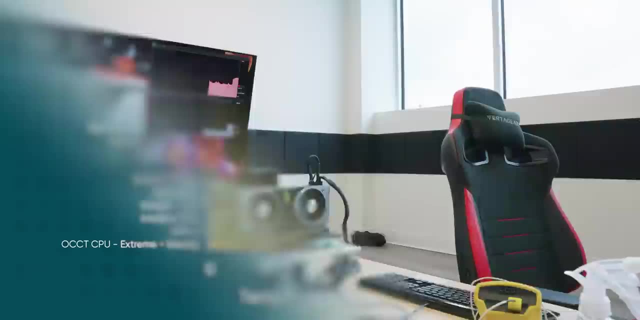 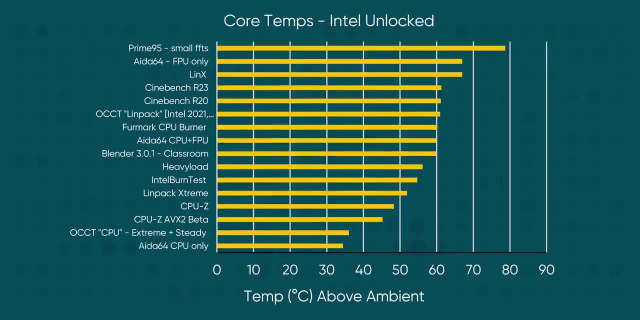 Turbo Boost power management was bunging up the other tests or something. we re-ran the entire suite with our Volt and our clock speeds back to stock and to say I'm shocked would be putting it mildly. It was like witnessing a brutal beatdown in slow motion Again. 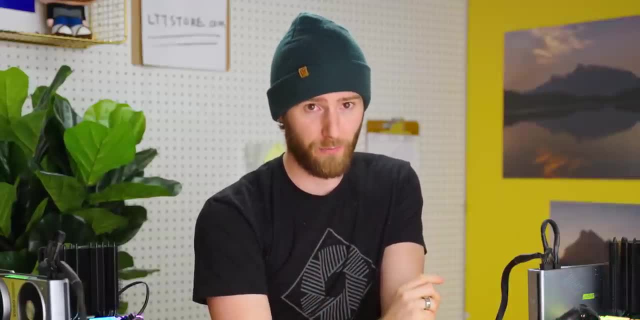 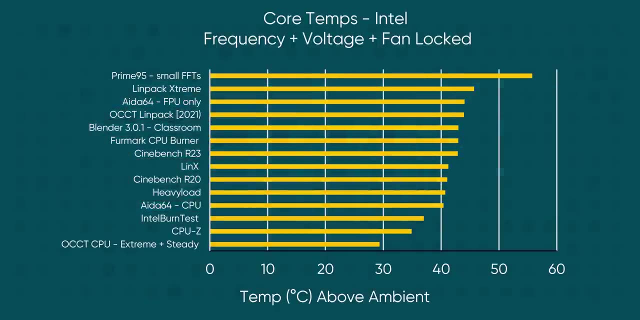 We have some theories here, but first let's get to the rest of the results. Our 10 middle performers had just a 6 degree overall spread. Then we had our underperformers: Intel Burn Test, CPU-Z and OCCT's CPU Large Dataset Extreme Benchmark. 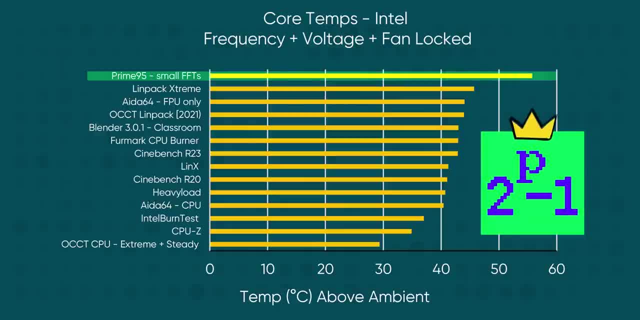 Then we had our underperformers: Intel Burn Test CPU-Z and OCCT's CPU Large Dataset Extreme Benchmark. At this point you can probably see why we declared Prime95 best in heat. but looking at thermals alone would be a huge mistake. 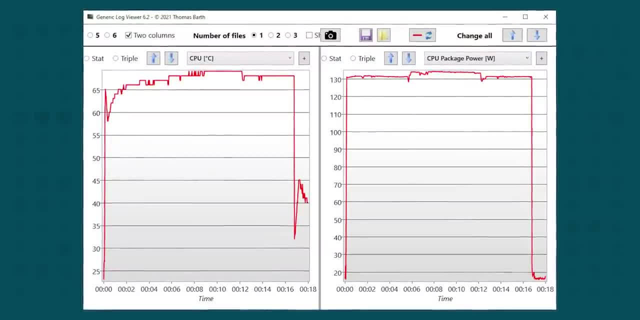 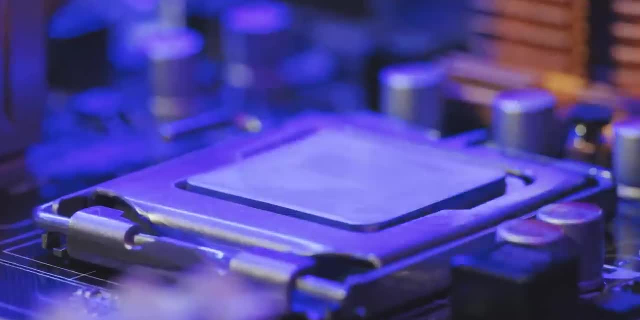 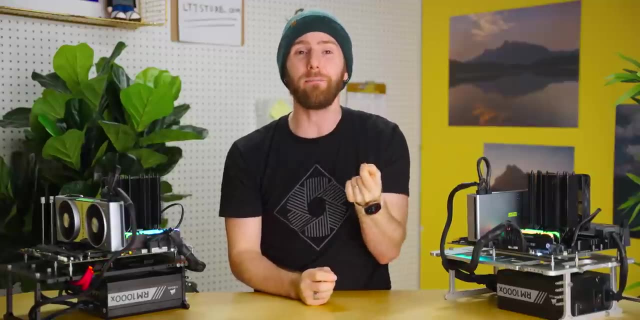 Check out the heat profile and power consumption profile of Prime95 Small FFT. Huge spikes, then they just hold indefinitely. It achieves this by repeatedly performing demanding mathematical calculations, but on a dataset that's so small it fits right in the CPU's on-die cache. 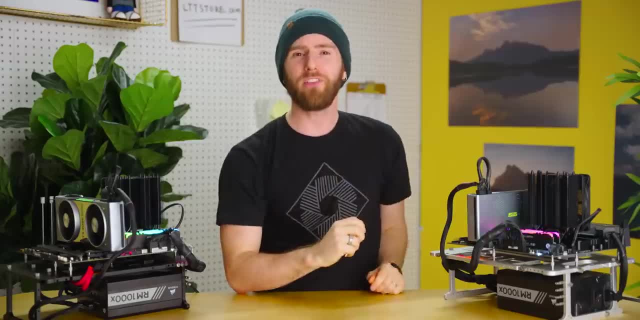 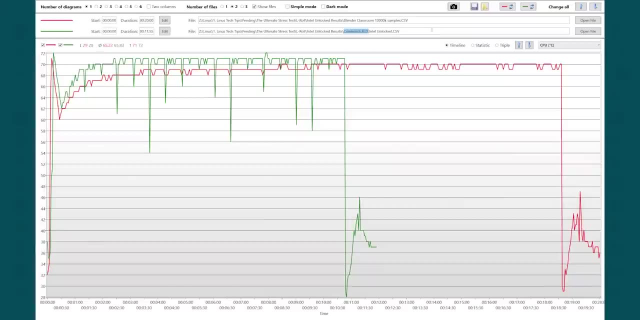 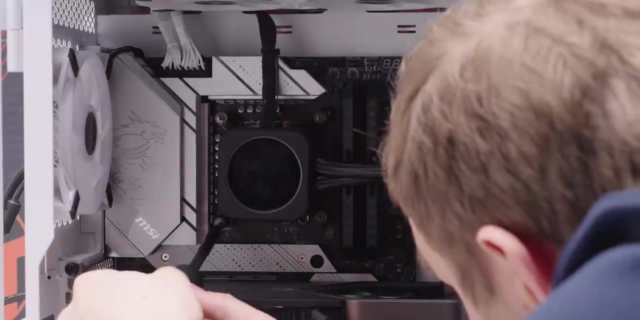 No bottlenecks, MAXIMUM BOTTLENECKS, But obviously no real-world application behaves like that. Even notoriously demanding professional workloads like CPU rendering in Blender or video encoding will generate very different profiles. So if I was validating a thermal design for a demanding client, 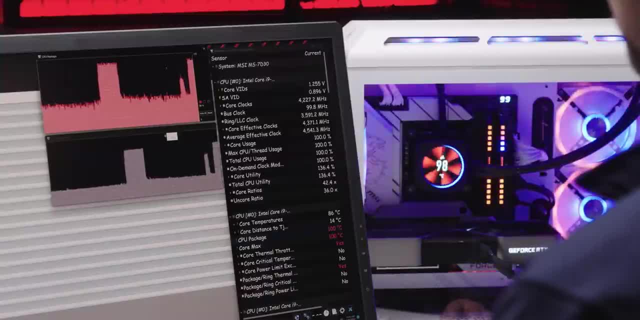 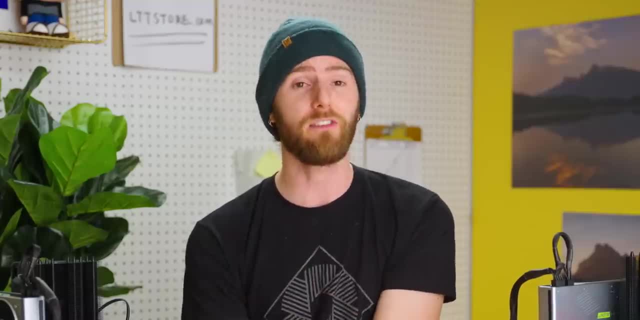 and I wanted to see an absolute worst-case scenario. Prime95 needs to be part of my toolkit, But if I care more about stability in real-world applications, I need to look elsewhere. Enter LINPACK, The most used stability stress testing tool of all time. 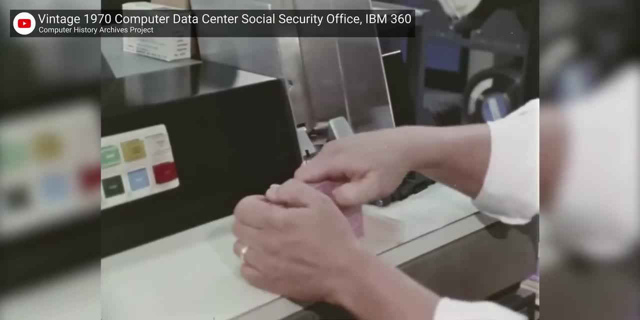 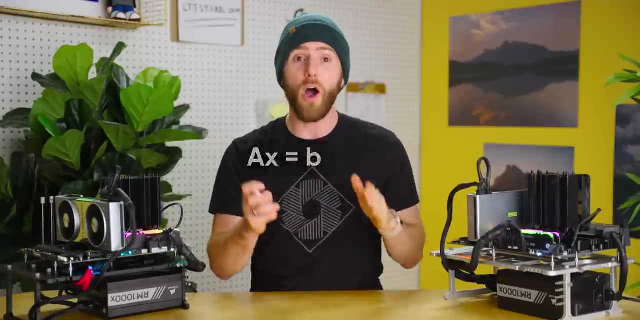 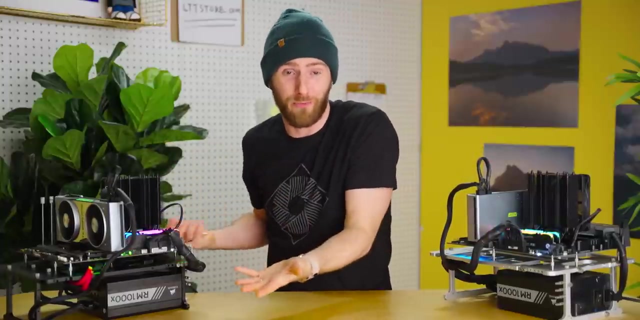 It was originally created for use on supercomputers in the 1970s And, in a nutshell, it's a software library that performs linear algebra. this equation specifically on repeat And it still behaves the same way today, Except it's been rehashed multiple times to keep up with modern computers. 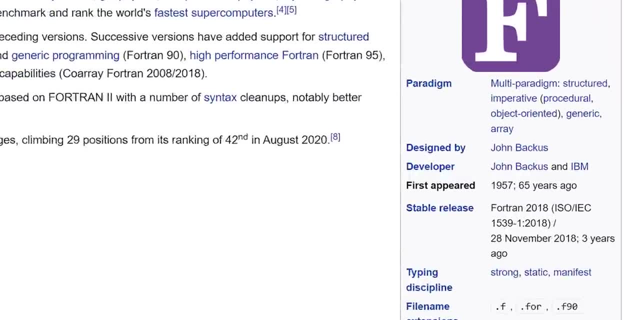 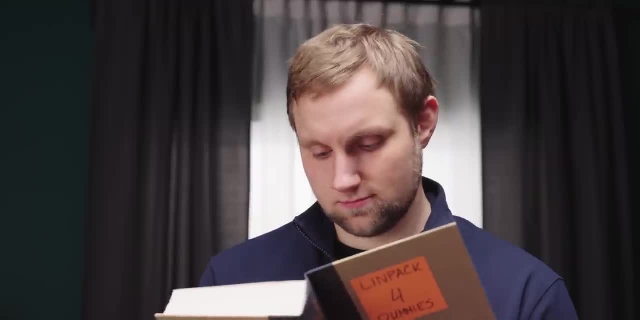 which is pretty important, considering that it was written in FORTRAN, a code language that is so old. it was originally input via punch cards. Fun fact, by the way. Because LINPACK is a library, not an application, it's easy for developers to integrate it into their own test suites. 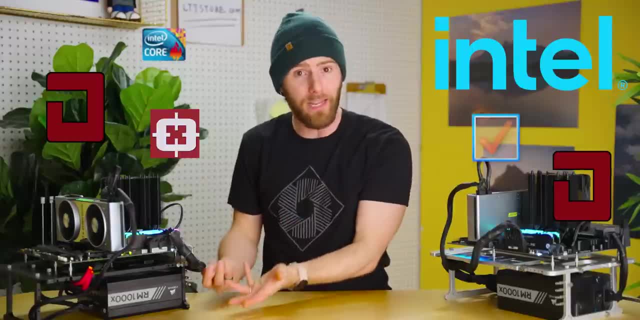 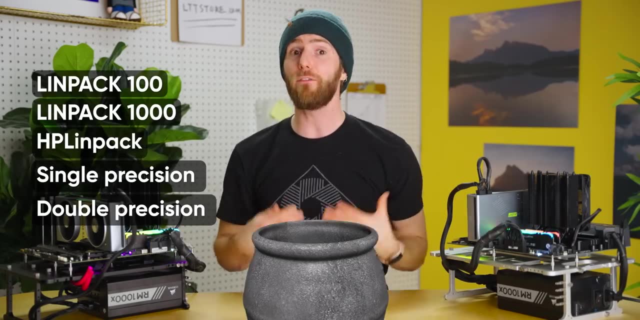 And six of the tests we used are actually LINPACK-based. But even then, not all tests are equal, because there are multiple LINPACK versions and any of those can be combined with other methods to create a complete hodgepodge of stress for your poor CPU. 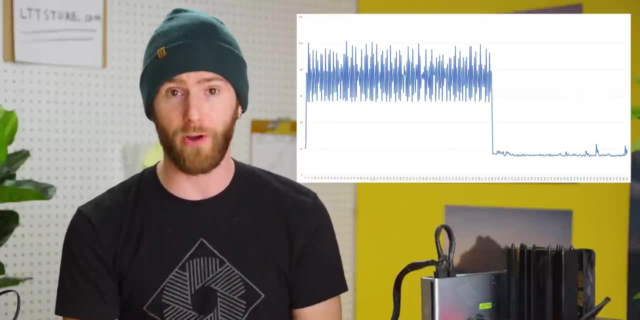 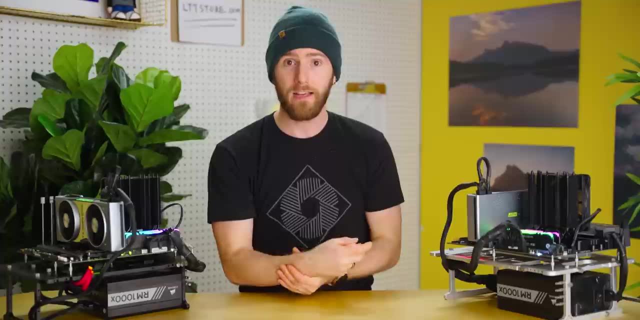 This is what a LINPACK load looks like on our thermal graphs: A spiky wave gets produced as each equation is solved, then there's a brief pause between calculations, And now that we know this, it's really easy to spot this shape in many of the tests that we ran. 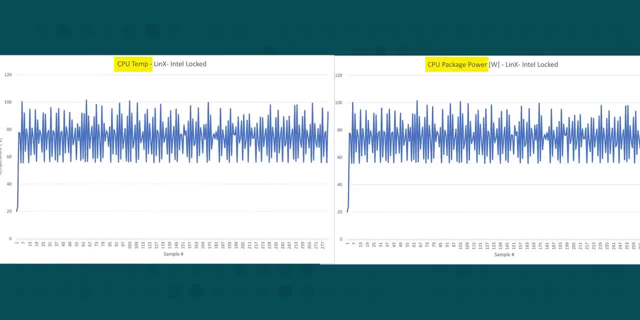 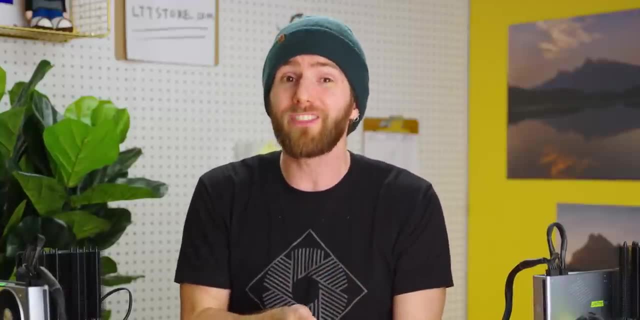 Now, if we switch from temperature to power consumption, we see well the same thing. These swings in power are really tough on not just your CPU, but also your motherboard VRMs and your power supply, which is a perfect combination for evaluating stability. 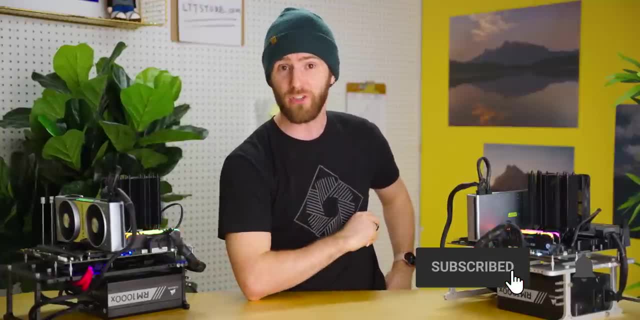 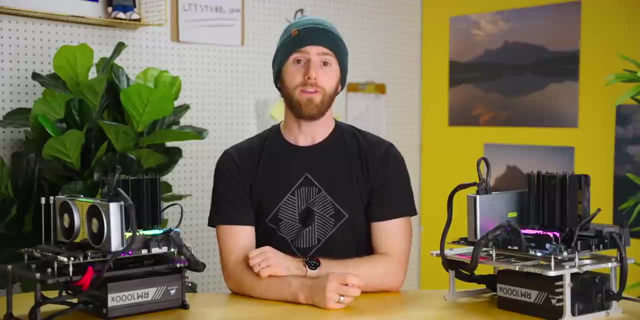 which we're definitely going to check out on AMD's 3D V-Cache CPUs. so get subscribed so you don't miss it. Also, buy a shirt or a water bottle- Haha, lttstorecom. On that note, let's take a look at our AMD results. 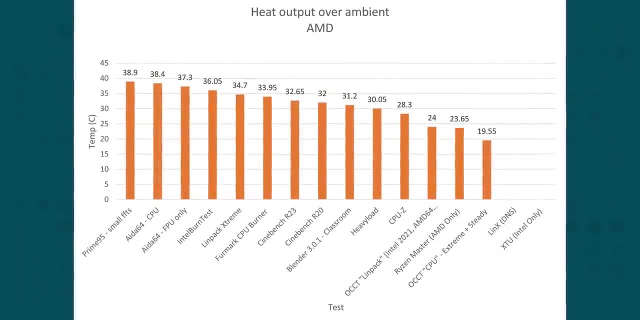 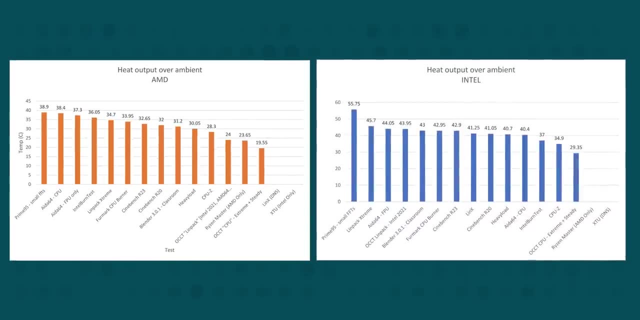 Here we didn't see anything that seemed anomalous, so we left our voltages and clock speeds locked per our original test methodology. To start with, AMD ran much cooler overall with delta Ts, so that's the temperature difference between ambient and our CPU. 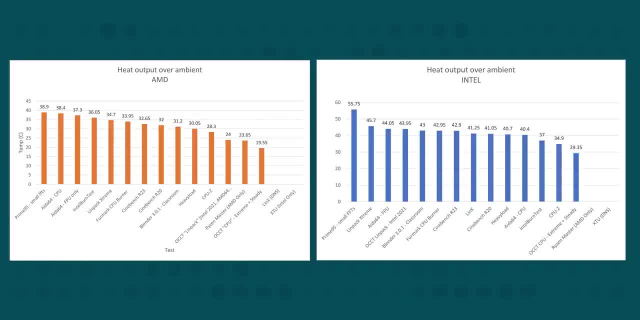 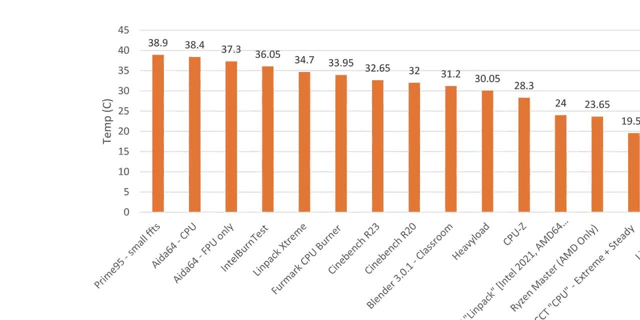 peaking at just 39 degrees compared to Intel's 56.. Man 12th gen performs, but, lordy, is it ever hot? Now? Prime95 still came on top for thermal stress, but only barely just half a degree behind was AIDA64. 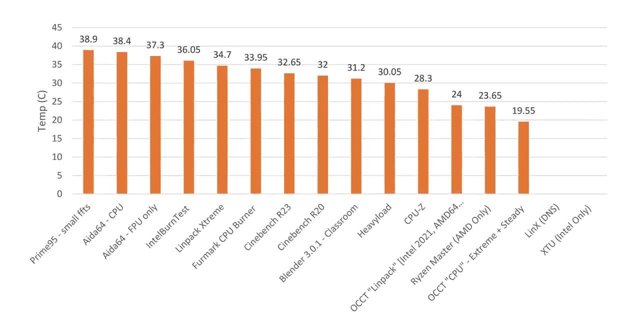 Then the middle of our chart doesn't have the same flat middle zone as Intel. Instead, there's a fairly consistent decline with a spread of about 10 degrees. Note, by the way, that Ryzen Master did run, but it's right near the bottom of these thermal stress loads. 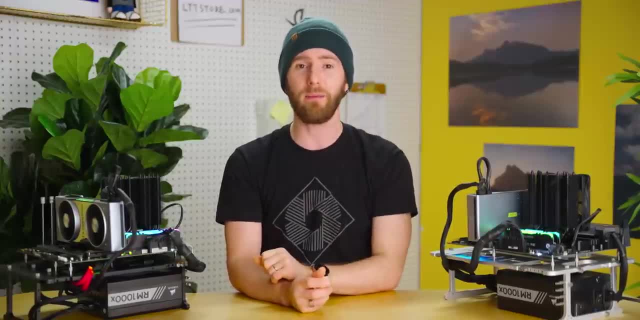 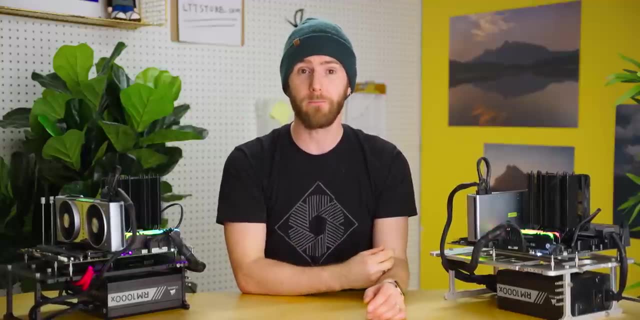 We don't know for sure why that would be, but my tin foil hat says that maybe AMD doesn't want you to cook your CPU. I don't know. though Even ignoring Ryzen Master, we can draw some interesting conclusions here. If you want to hit it hard, it's Prime95 for maximum heat output. 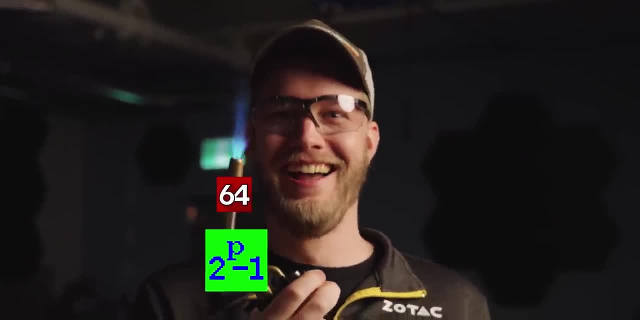 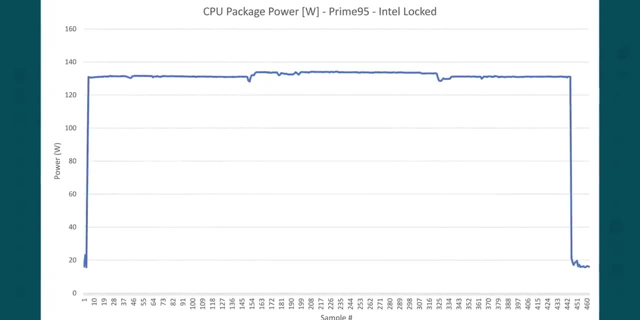 with AIDA64 FPU as a close runner-up. As for stability, well, we already learned that this is not what we're looking for. We want a rapidly oscillating power load, so let's have a look at one of our LINPACK loads: OCCT, LINPACK 2021, and oof. 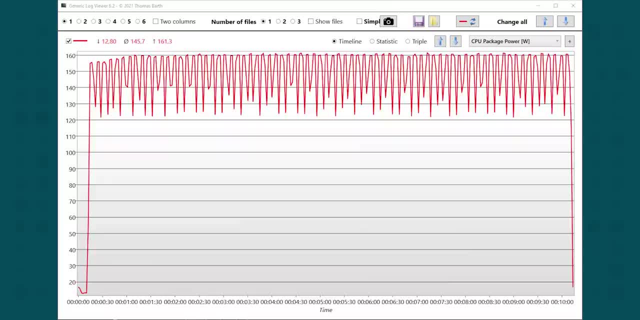 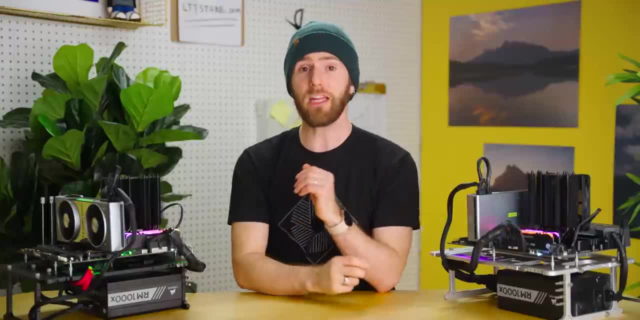 Look at that power draw porcupine right there: 35 watt spikes, roughly 6 times per minute. How about LINX? Again very nice, Very stable clock speeds, which we expect since we locked it. but we still saw some intermittent clock drops. 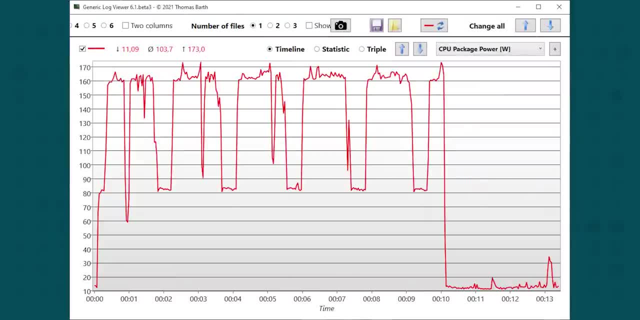 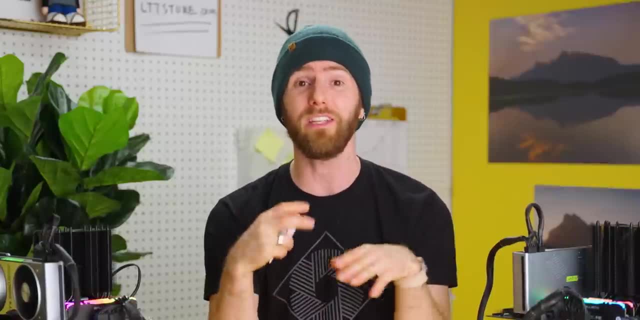 and huge swings in power draw from 82 watts all the way to 170 watts. This is probably the best example we could have hoped for to show you why you need to test with multiple pieces of software. So let's take a look. 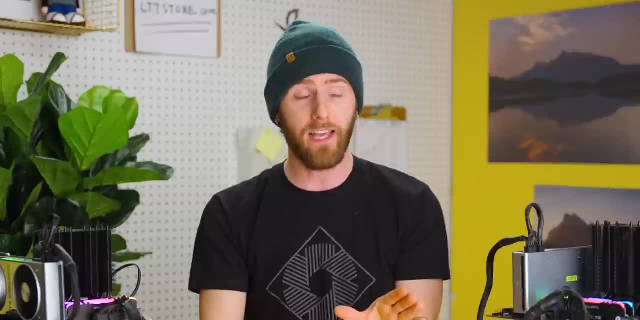 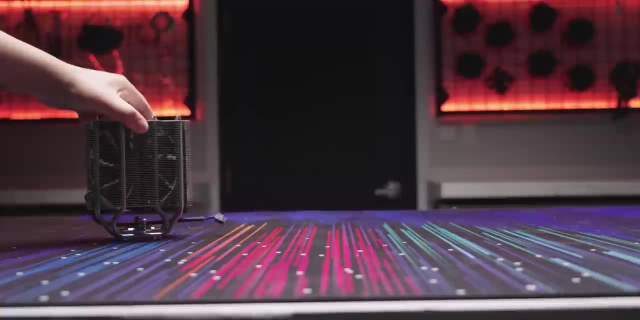 Every one of these is a valid part of your stress test toolkit, Yet each is different. Sitting down and inspecting these results, though, lead to some pretty tidy conclusions for you to take with you If you want to get in and out quickly. 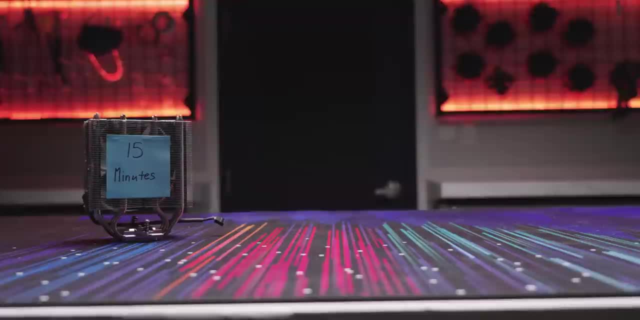 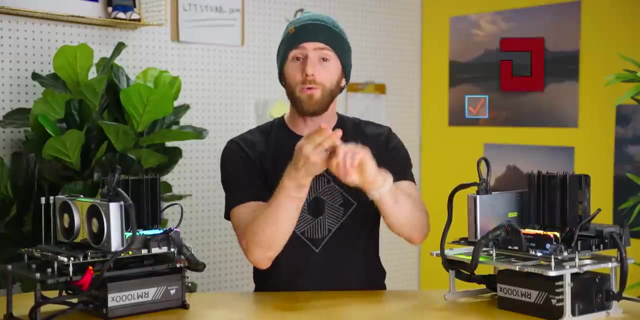 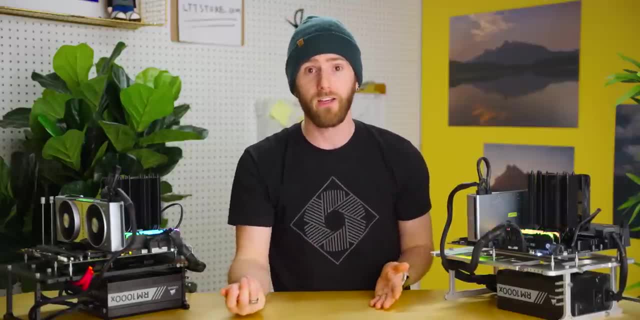 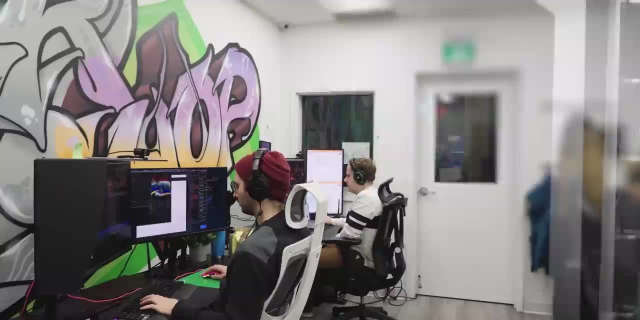 for how long you need to run them, though, because it comes down to personal preference. For a gaming test bench, I might be comfortable with 10 minutes, But for a video editing workstation that I want years of service from 24 to 48 hours isn't out of the question. 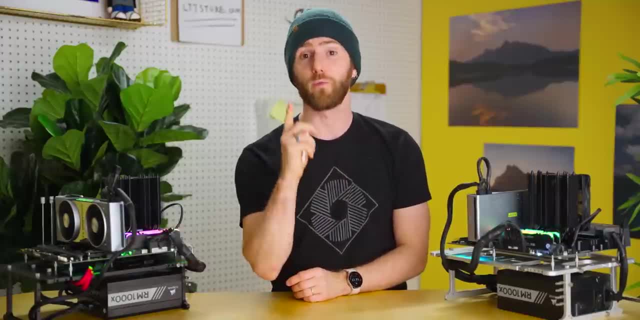 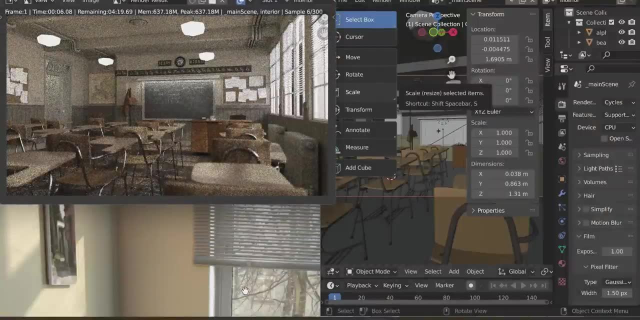 Also, none of these synthetic loads excuse ignoring real-world ones. If you've got the time and if you're serious about it, a blender render or a continuous Cinebench run followed by a few rounds of PugetBench would absolutely be a good idea. 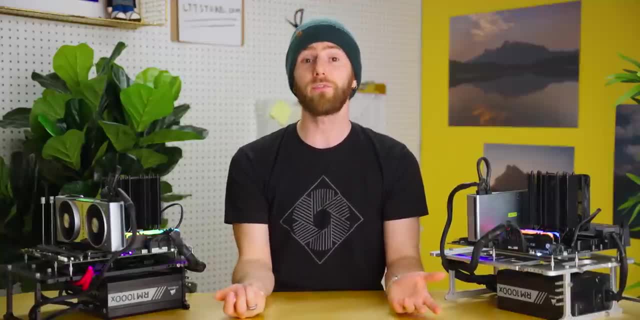 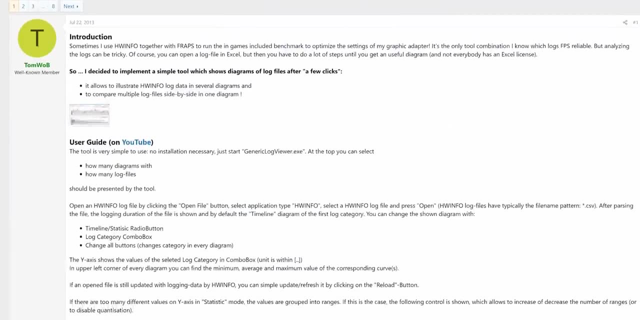 Now it may not be common knowledge, but the tools that we use to log and review our data today are both free for personal use- HWinfo and Generic Log Viewer- and you can check them out at the links in the video description. HWinfo allows you to log all your sensor data. 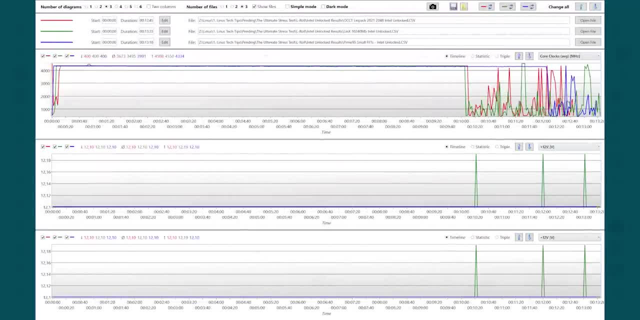 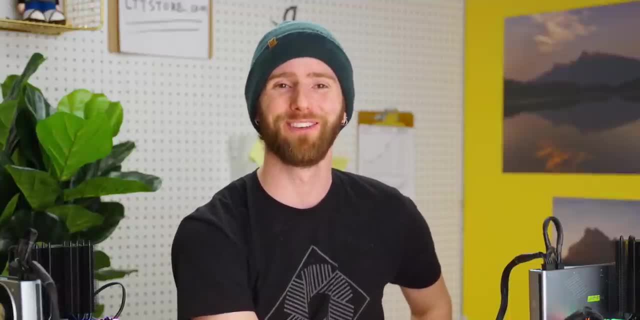 while Generic Log Viewer gives you a perfect tool for quickly and easily charting that data and comparing against other runs. What I hope is common knowledge, though, is our sponsor, Micro Center. Micro Center is one of the best places to shop for desktops, laptops, computer components, monitors. 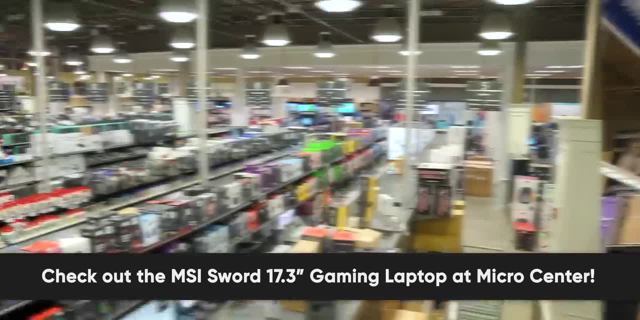 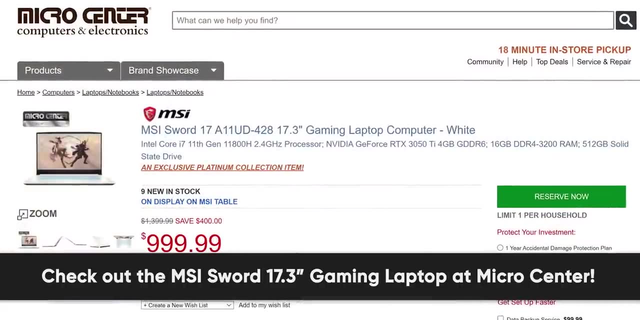 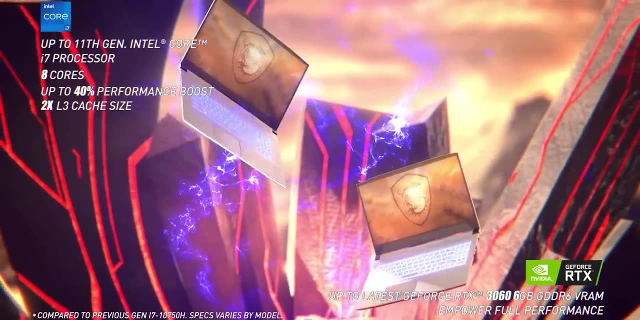 TV networking equipment and all your technology needs. They've got great prices and great selection and 25 locations across the US. You can check out the MSI Sword 17.3-inch gaming laptop at Micro Center featuring an Intel Core i7-11800H, NVIDIA RTX 3050 Ti graphics. 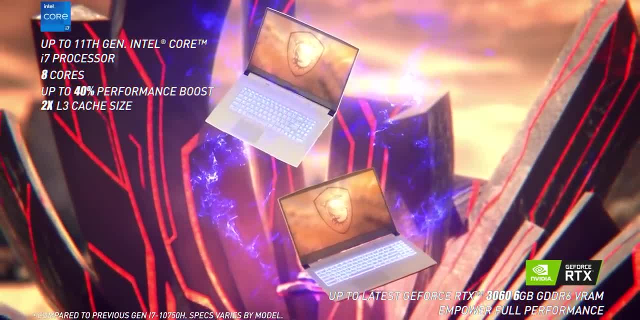 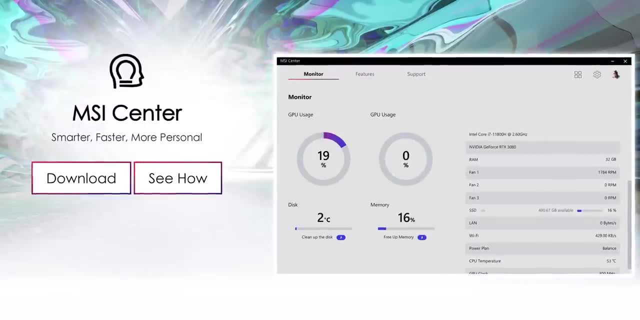 16 gigs of DDR4 RAM, a 512-gig SSD and, of course, a 17.3-inch 144-hertz IPS display. Plus, the MSI Center app helps you easily control and customize your laptop for different use cases.